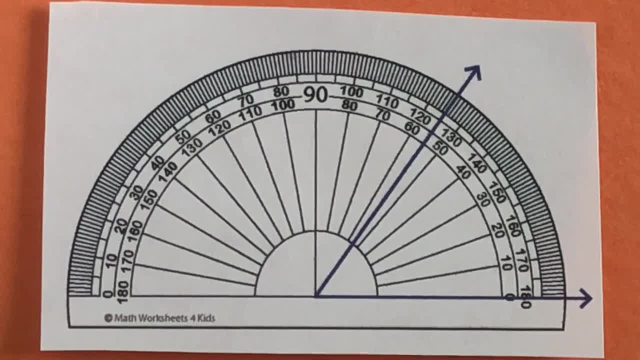 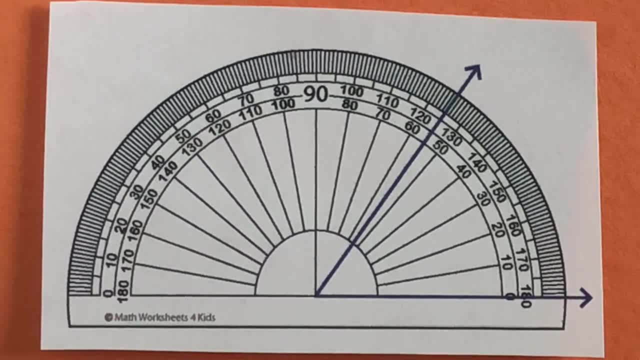 week. They were actually pretty good. There were still some mistakes, and mainly the mistakes that are being made are reading the wrong numbers, which is always the trickiest part of reading a protractor. So I just want to go through that again very quickly with you. All right, let's take 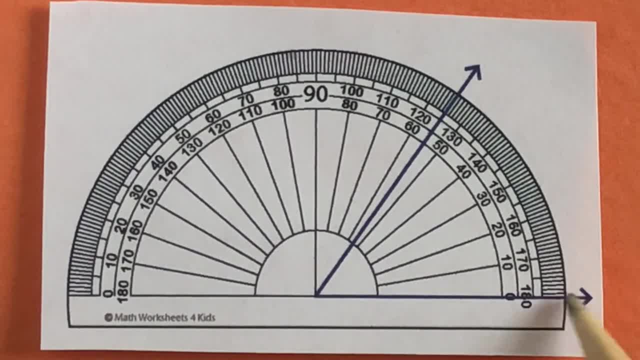 a look at this first protractor right here. All right, here's our angle. You can see it measured there. All right, I can look at that angle and I should right away be able to say that's an acute angle. So I'm going to be looking at the smaller numbers. That's my first way I like to do it. 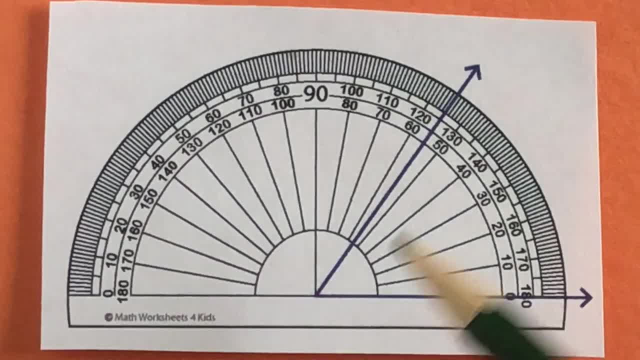 All right. my next way I look is I say: okay, here is the baseline of the angle, That means what's laying on that flat line there. Okay, it's the array that's laying right there, And I see that that's the zero starts here. So I'm going to be counting this time those inside numbers. This is: 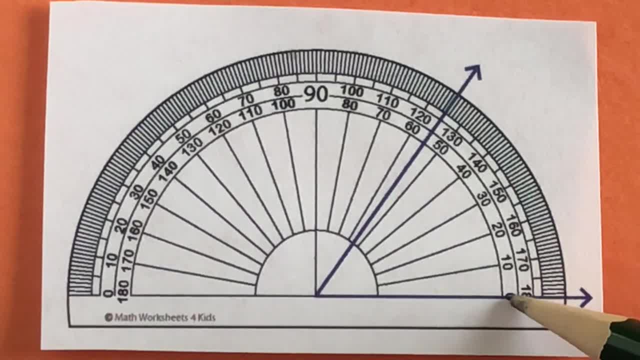 the ones I always think are a little harder to count because we're counting backwards. All right, so I'm going to go through and I see 0,, 10, 20,, 30,, 40, 50. And then so it's between: 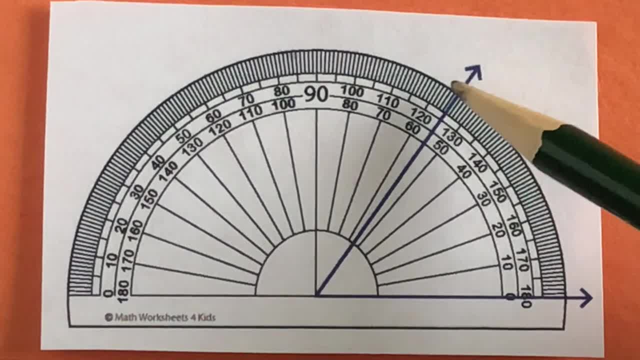 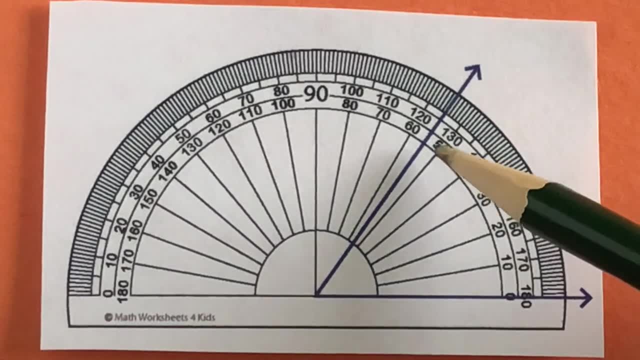 exactly between 50 and 60. All right. Now I don't want to be confused by this 120 and 130 up here, because that's the obtuse measurement, if the angle there, So it's between 50 and 60.. All right, Some. 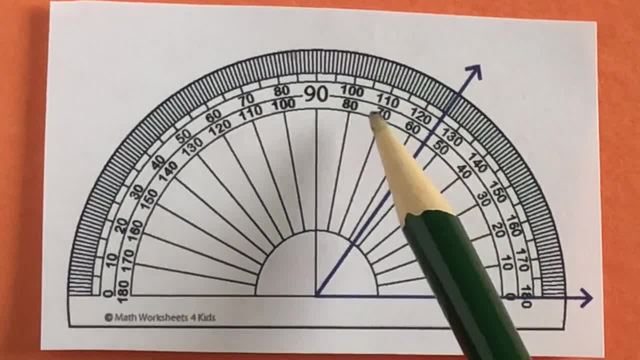 people naturally want to read this as 65. And the reason is is because, look you see, oh, here's 60. What comes after 65?? But remember, the inside is always backwards, So we're going to call this. 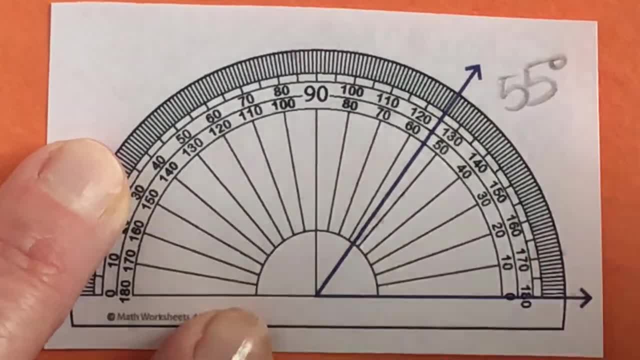 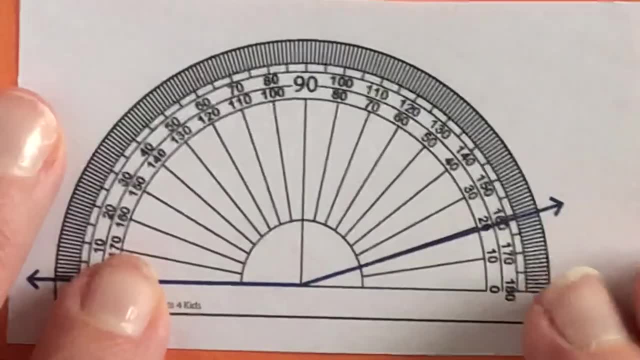 one right here, 55 degrees. Okay, so that's our first angle, And then we're going to go through the first one there. All right, let's take a look at our next one. Okay, our next angle here. Oh, 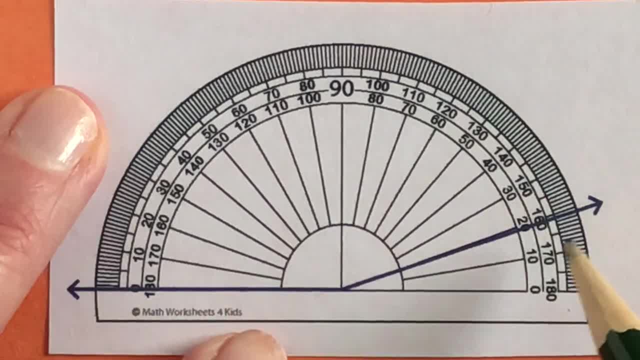 this is a big, giant, obtuse angle. All right, So now we're going to be definitely looking at bigger numbers. Here is that baseline of the angle, right here that ray that's laying right on the black line, And that's our zero. So you can tell, we're going to be reading those outside numbers And we 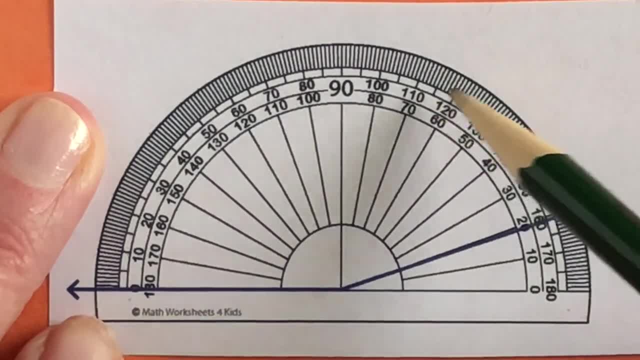 definitely want to read the bigger ones. Okay, so I'm going to go around, start reading them. Here's 150.. Here's 160.. And then we're going to go through the outside numbers, And then we're going to go. 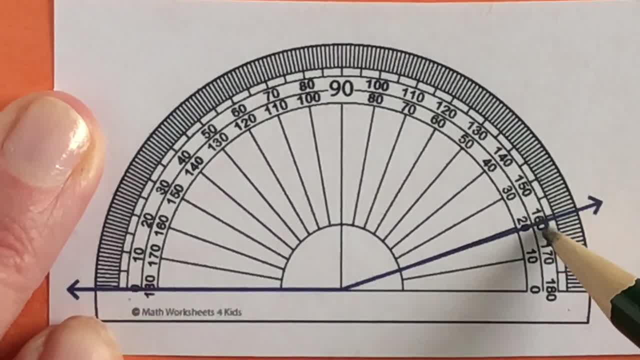 160.. Here's 170.. Okay, so it's almost right about 160. But if I look super close I can see that it's about one space after 160.. So one more than 160 would be. you got it 161 degrees. Now, if you. 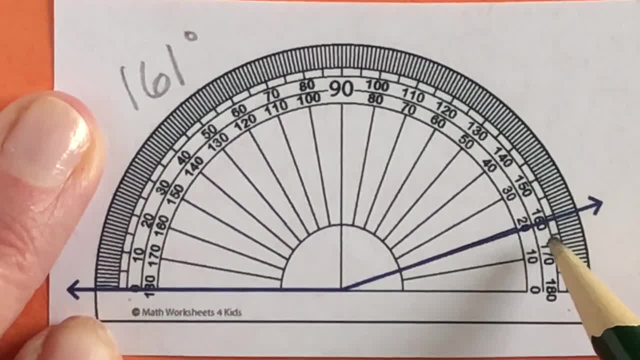 were to mark this as 160 on a test, it would still be fine. I would still give you credit for that, as I'm sure any teacher would, because with using protractors it's kind of like one or two either way of what the angle actually is. 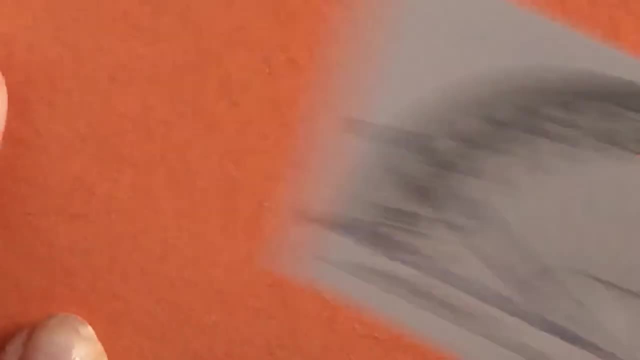 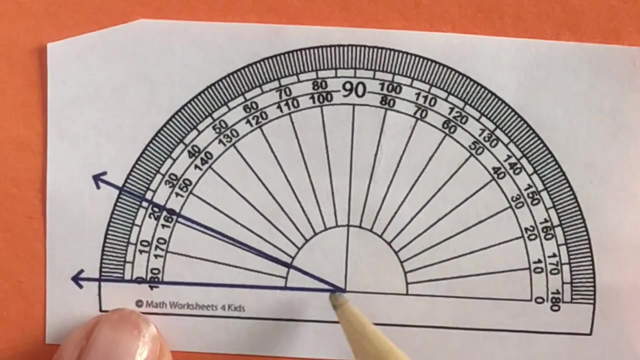 Okay, so that one's 161.. Let's take a look at our next one. Okay, here is our next. Oh, this is a little acute angle. All right, that baseline of the angle is over here. So here starts our zero. 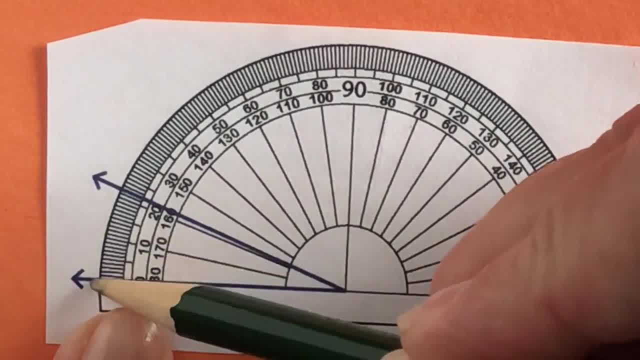 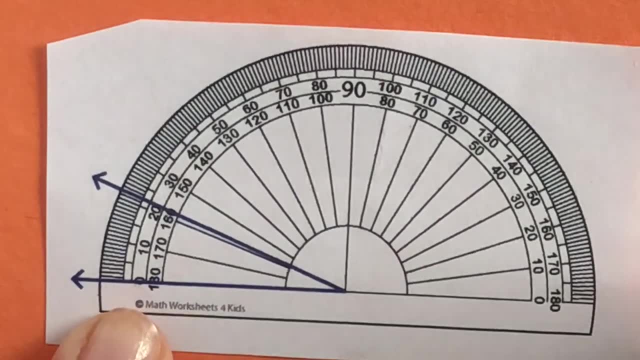 It's definitely acute. We want small numbers, So we're going to go up the side. We're going to read: Here's 10.. Here's 20.. To me that looks like it's about two past the 20.. So I'm going to call. 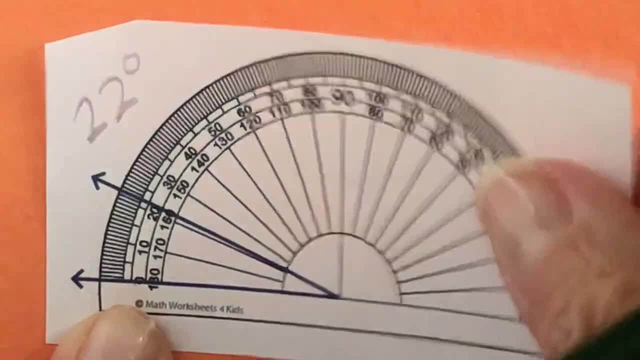 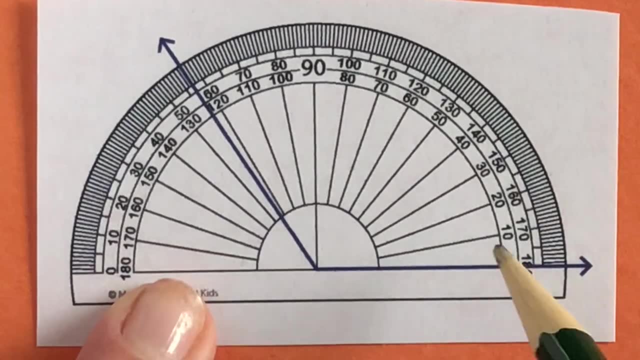 it 90 degrees, All right. again, I don't want to read those big numbers because it's not obtuse. All right, and our last one we're going to look at is this one: Okay, so it's a big obtuse angle. 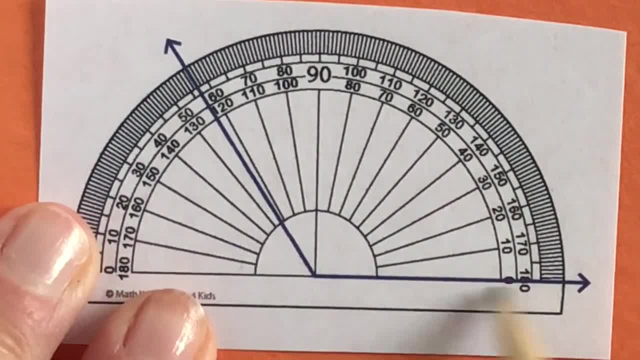 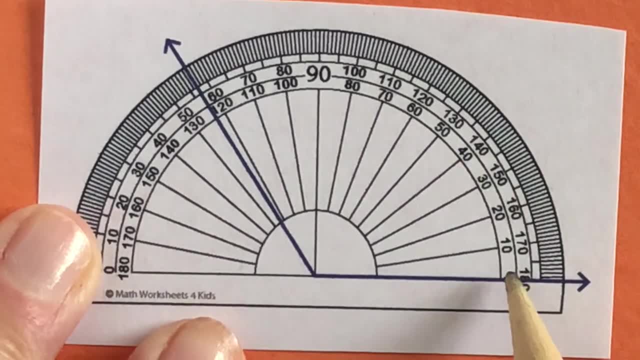 bigger than 90 degrees. Okay, here starts the baseline, right here at the angle. Okay, so here's our zero. So I'm going to read these insides And remember insides, read backwards. Okay, so I'm going all around, all the way around. So here's 120.. 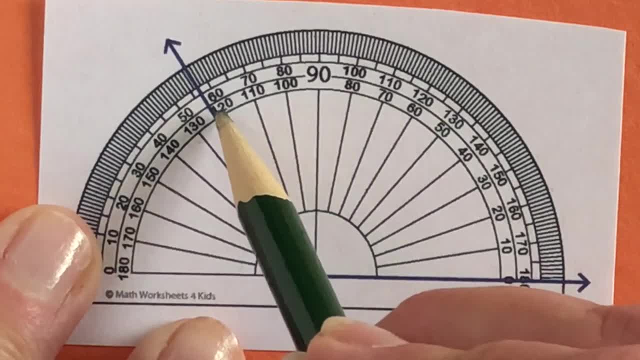 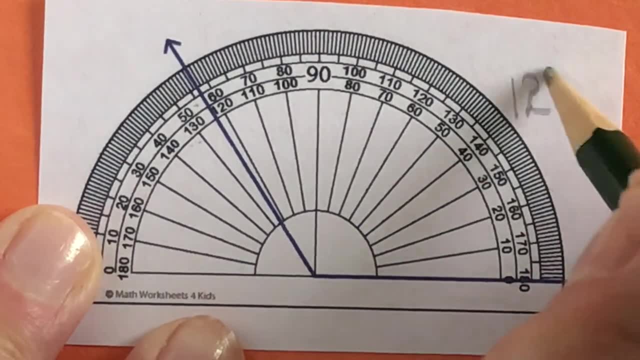 It's on the way to 130.. Okay, so it's after 120.. And it's not quite this little tiny line up there, you can see is 125. So I'm going to actually call that one about 123 degrees. Okay, so that's the. 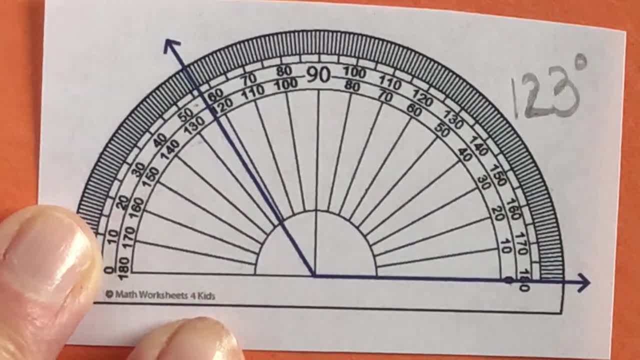 way we're going to do these Now. boys and girls, you're going to have a slideshow this week in Schoology that's going to practice a few of these types of problems and the few we're going to do next. So if you watch all the videos first, then go through and do the slideshow. That'll be the 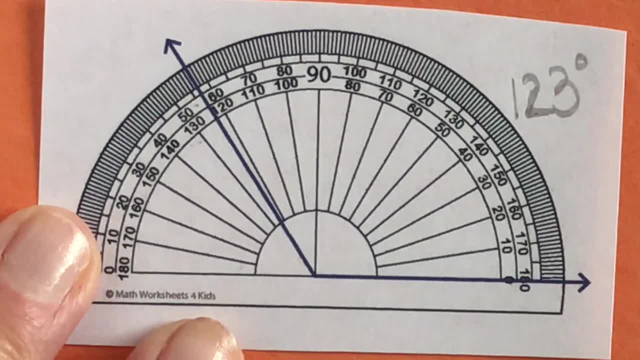 easiest, And then later this week we'll have a short quiz. Do these things just to make sure you're understanding correctly. Okay, that's all for this video. We'll see you in the next one.